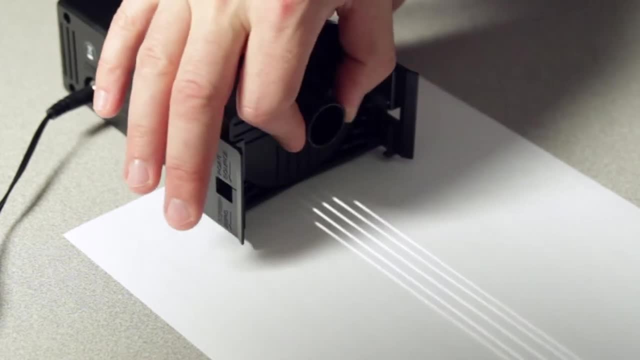 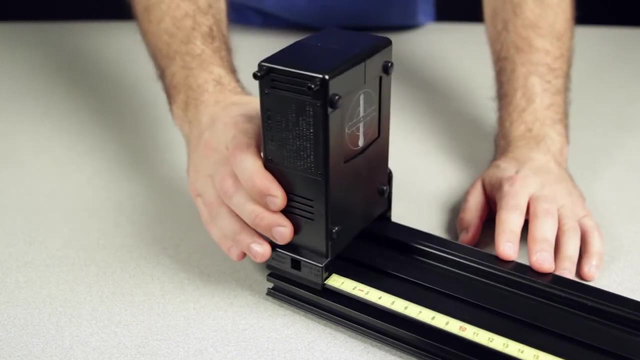 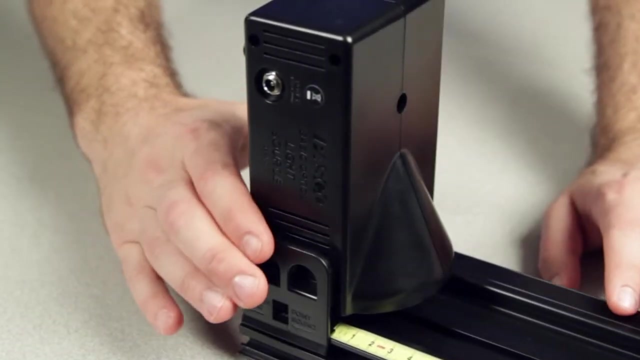 color source or a ray box with up to five parallel rays. To mount the light source to an optics track, place it vertically on the track and press down The outer tabs of the light source. snap into the side slots of the track To detach the light source, squeeze the release lever and pull up. 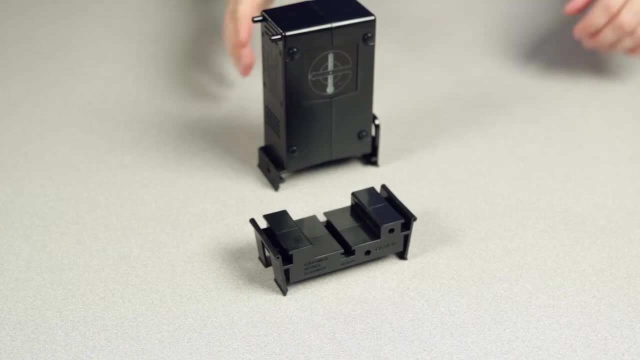 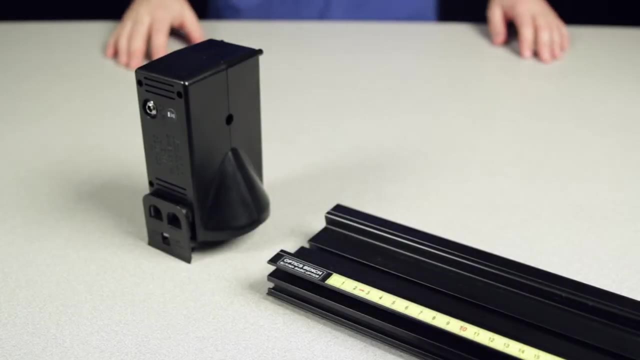 Similarly, the light source can be mounted to a Dynamics Track Optics Carriage by placing it in the center of the carriage and pressing down to snap it in place. To use the light source as a point source, mount it vertically on an optics track or. 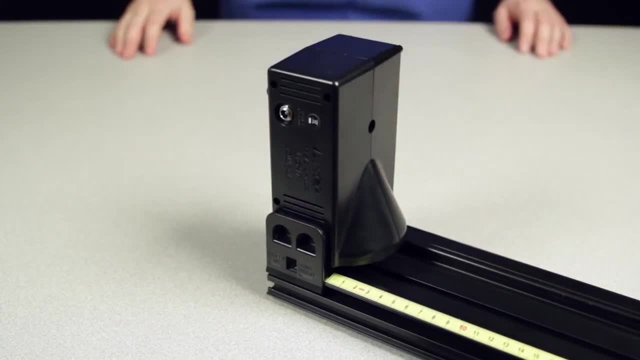 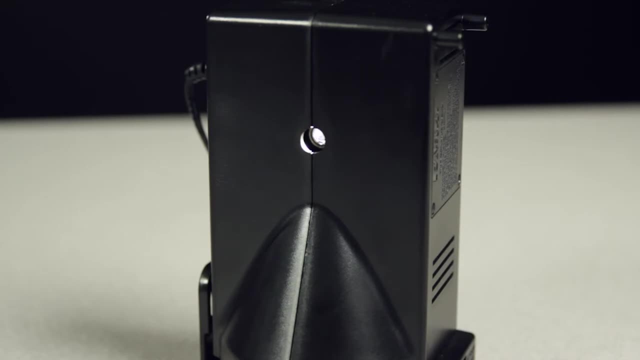 carriage with the point source opening facing down the length of the track. The Halogen Bulbs filament closely approximates a true point source by projecting light through the round opening in the case, but its actual location is about 3 cm behind the outer surface. 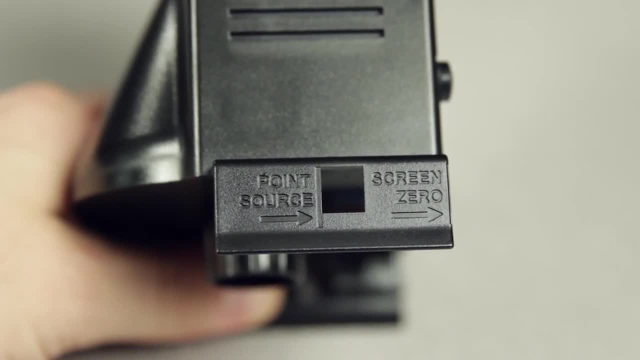 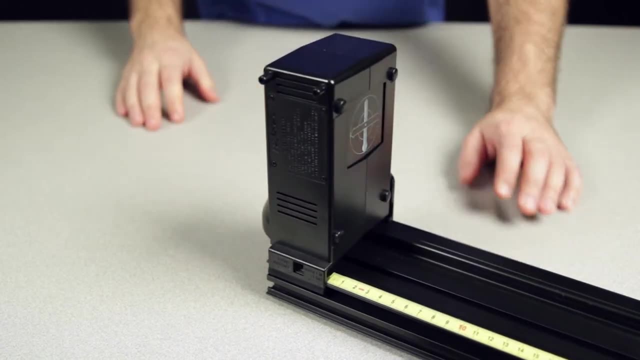 of the case, as indicated by the marks on the tabs. To use the light source as an illuminated object: mount it vertically on an optics track or carriage with the crossed arrow target facing down the length of the track. To use the light source as a point source: mount it vertically on an optics track or 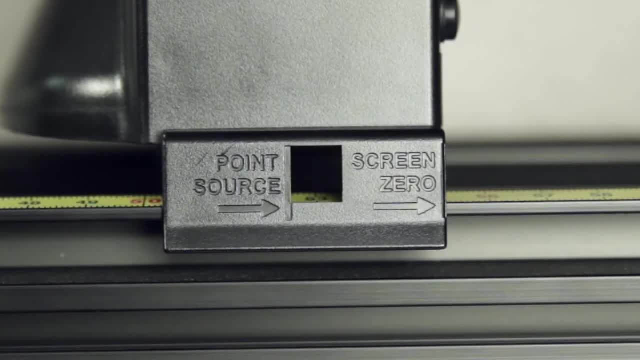 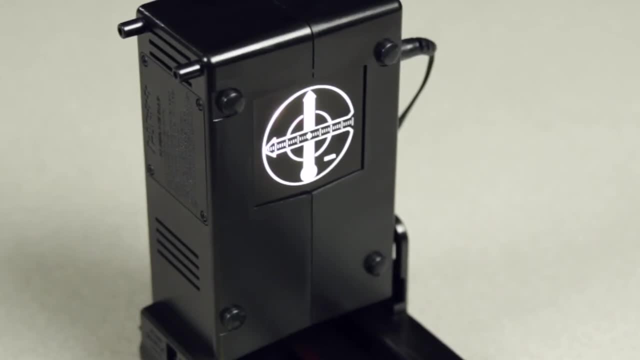 carriage, with the crossed arrow target facing down the length of the track. Marks on the tabs at the base of the light source indicate the horizontal position of the object's screen. The object is a backlit, translucent screen with crossed arrows printed on it. The pattern is asymmetrical, so you can tell if images. 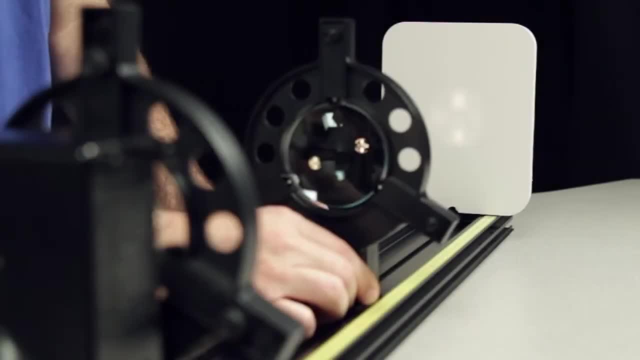 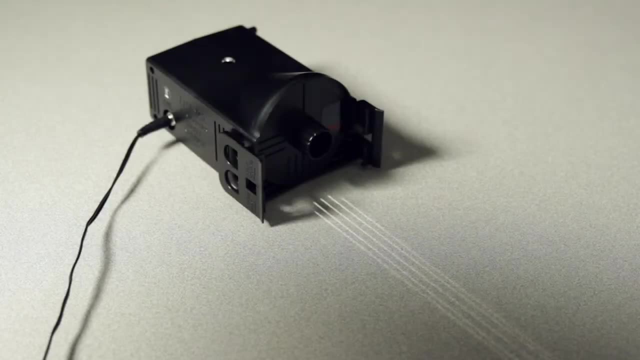 formed by lenses and mirrors are reversed or inverted. Millimeter scales on both arrows allow you to measure the magnification of an image even if the entire image is not visible. To use the light source as a ray box, place the unit flat on a tabletop. 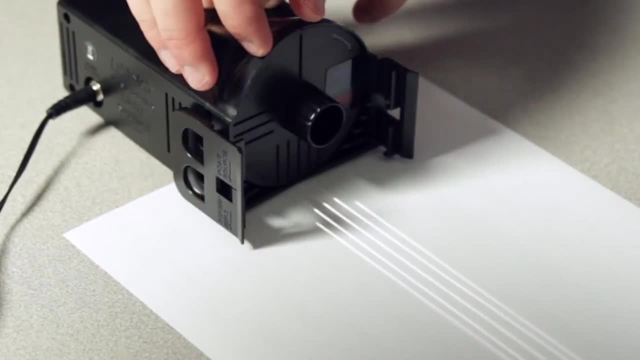 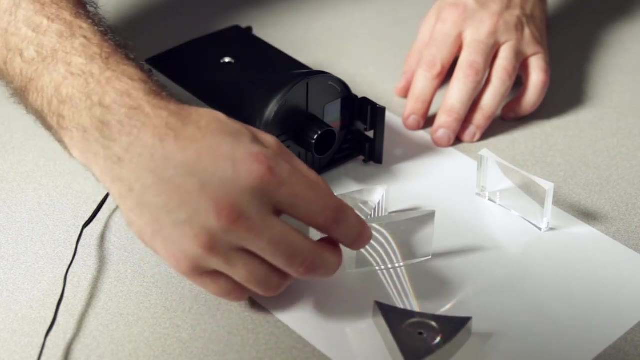 Use a wheel to select one, three or five parallel rays projected onto the table. A sheet of white paper placed flat on the table makes the rays easier to see and allows you to trace them with a pencil. Use prisms, mirrors and cylindrical lenses to study how light rays are refracted and. reflected.